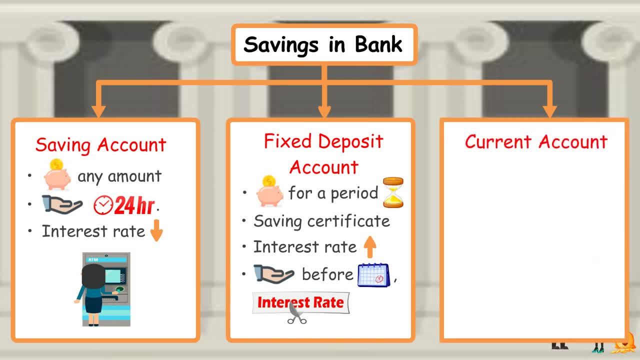 Number 3. Current Account. Number 3. Current Account. Savings can be used for personal or business purposes. Savings can be used for personal or business purposes. May make payment to another people by cheque. May make payment to another people by cheque. 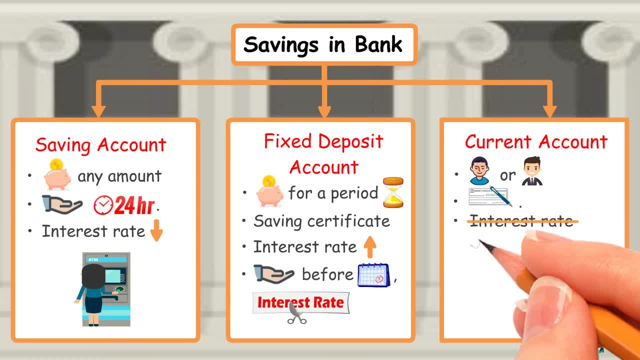 Savings will not be paid interest and need service charges. Savings will not be paid interest and need service charges. Savings will not be paid interest and need service charges. submit a referral. who is an existing current account holder at the same bank? Normal withdrawals: 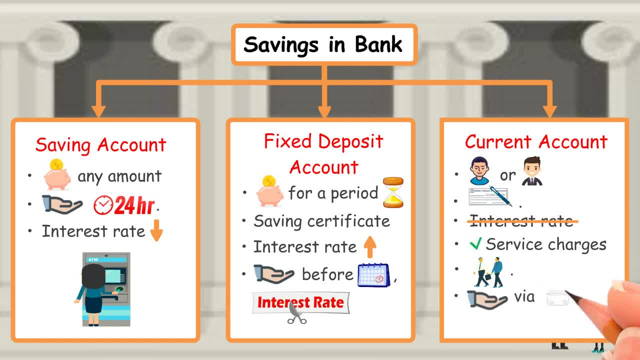 are usually allowed via debit cards and other channels, for example internet banking and telephone banking. It is an overdraft facility, which means can withdraw money beyond the balance of the deposit, but with interest charges. The benefit of savings is the interest for. 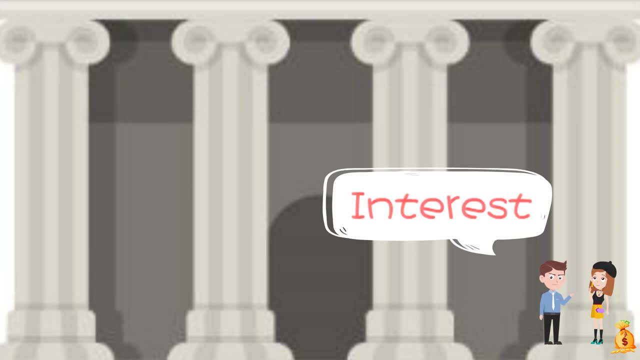 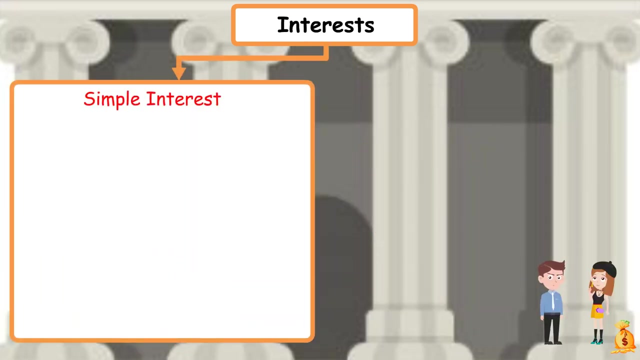 savings are rewards paid by financial institutions, for example banks, to depositors. There are two types of interest: simple interest and compound interest. Let's have a look at simple interest first. Simple interest is reward given to the depositor At a certain rate on the deposit amount principal for a period of time. 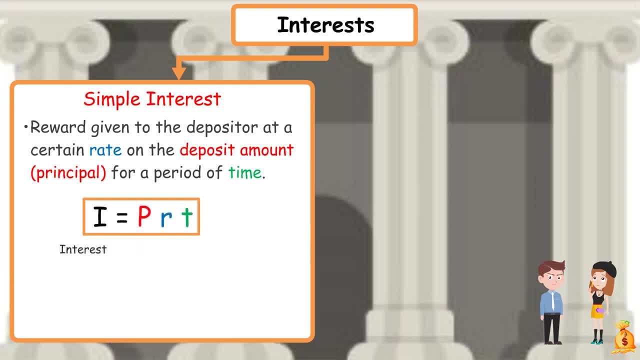 Formula is: I equals PRT. where I is interest, P is principal, R is rate and T is time. Take note: if rate given in percentage form, need to divide it by 100.. If time given in months, need to divide by 12 months. 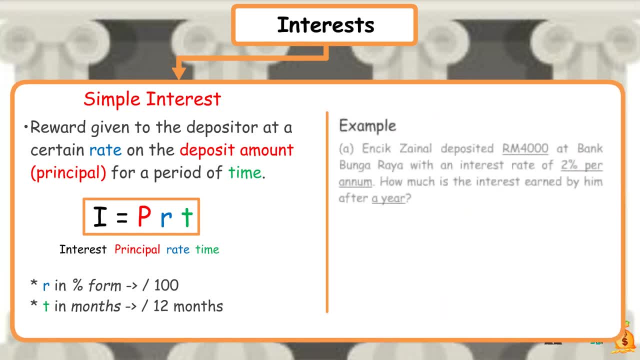 Example: A N6INL deposited RM4000. At bank Bunga Raya with an interest rate of 2% per annum. How much is the interest earned by him after a year? Base on the question principal is RM4000.. Rate is 2%, so is 2 one hundredths. 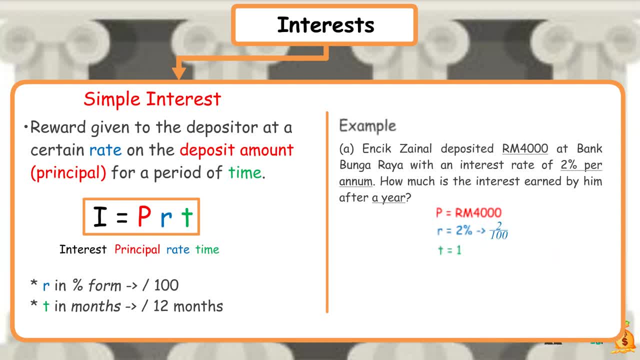 And T is one year. Write down the formula: I equals PRT. I equals RM4000 times 2, one hundredths times 1.. Say underscore 1 equals RM80. Therefore the interest is RM80.. Example B: Ms Wong deposits RM10000 in bank Moriney with an interest rate of 4% per annum. 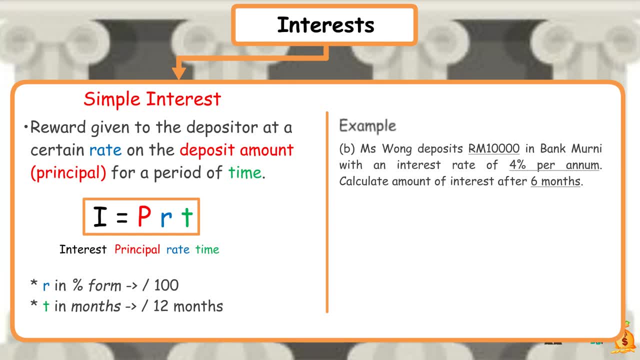 Calculate amount of interest after 6 months Base on the question. principal is RM10000,. rate is 4%, so is 4 one hundredths. Time is 6 months, so 6 twelfths. Write down the formula. I equals PRT. 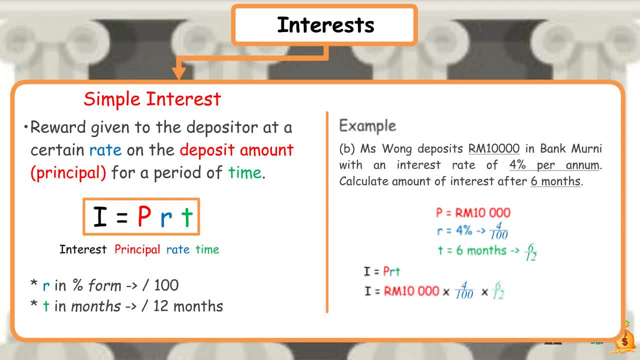 I equals RM 10,000 times 4 one-hundredths times 6 twelfths equals RM 200.. Therefore, the interest is RM 200.. For simple interest, the longer the saving period, the higher the returns. The higher the interest rate, the higher the returns. 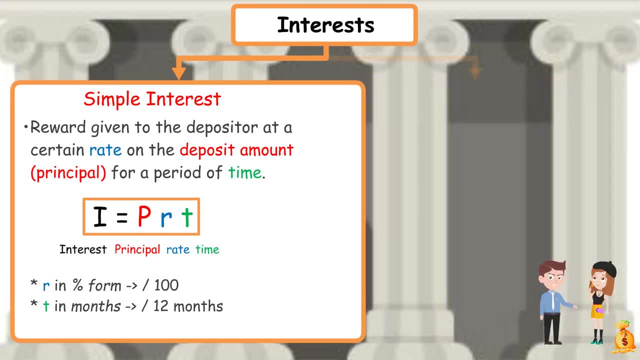 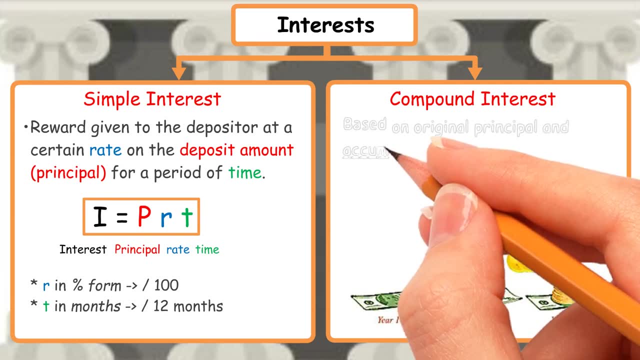 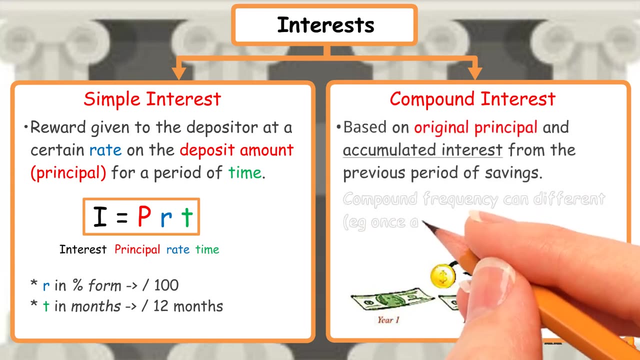 Second type of interest: compound interest. Compound interest is calculated based on the original principle and also the accumulated interest from the previous period of savings. Frequency of compounding on the principle can be different, for example once a year and once every three months. 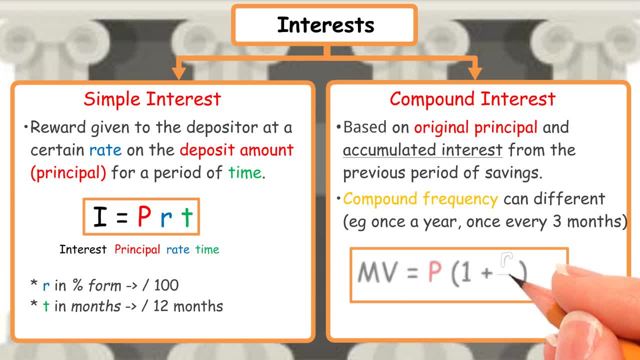 Formula: MV equals P. open parenthesis: 1 plus R over N. Close parenthesis to the power of NT. Where MV is matured value: P is principle, R is yearly interest rate, N is number of periods, the interest compounded per year and T is term in years. 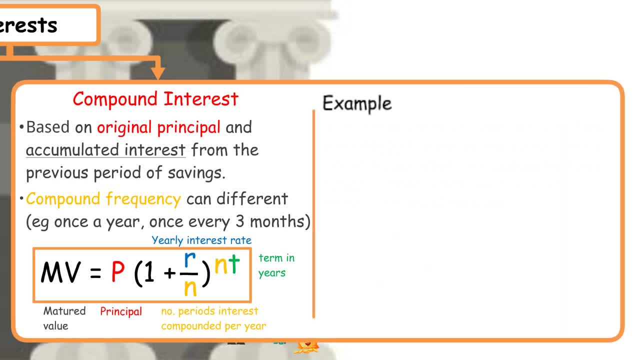 Example: at the beginning of a year, Mrs Liu Fang saves RM 15,000 in her savings account with a rate of 4% per annum and compounded every six months, What is Mrs Liu Fang's? Based on the question principle P is RM 15,000, rate R is 4%, so 4 one-hundredths equals 0.04.. 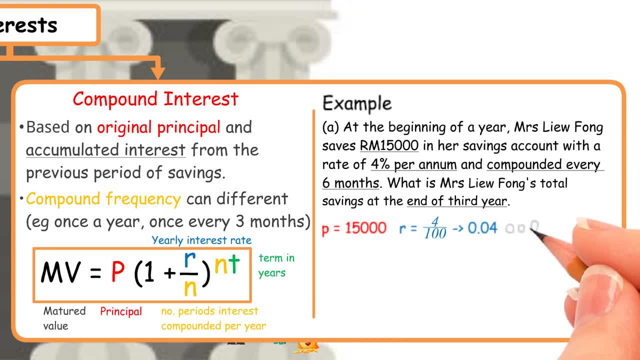 Number of periods, the interest compounded per year N is 2, and term in years T is 3.. Write down the formula: MV equals P, open parenthesis, 1 plus R over N. Close parenthesis to the power of NT: MV equals RM 15,000, open parenthesis, 1 plus 0.04 over 2.. 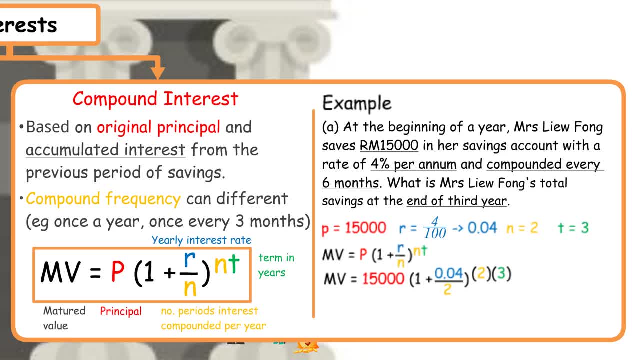 Close parenthesis to the power of 2 times 3.. Equals 15,000 times 1.1262.. Equals RM 16,892.44.. Therefore, the matured value after three years is RM 16,000.. 6,892.44.. For compound interest: the higher the compounding frequency, the higher the future value. 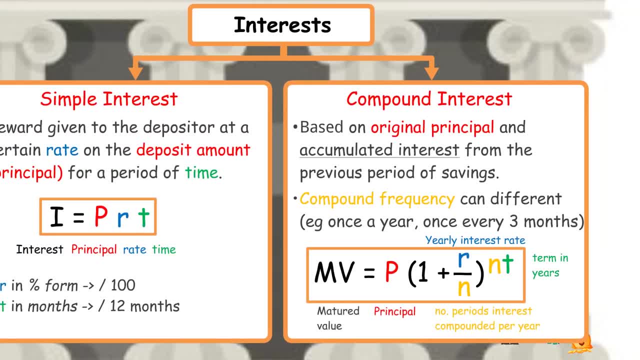 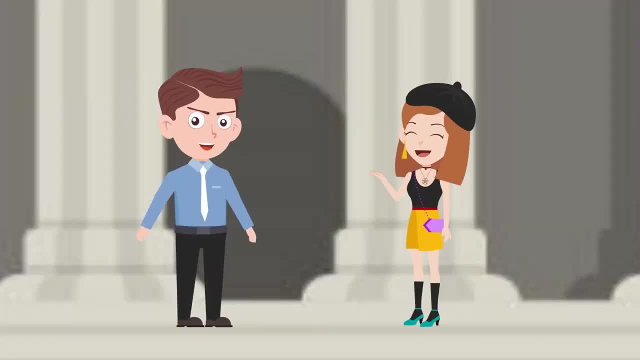 of savings. Savings with compound interest give higher returns than simple interest. Thank you, Mr David. Now I understand what are the saving accounts in bank and how to calculate the interests. By the way, I heard there is something called Islamic banking. do you know it? 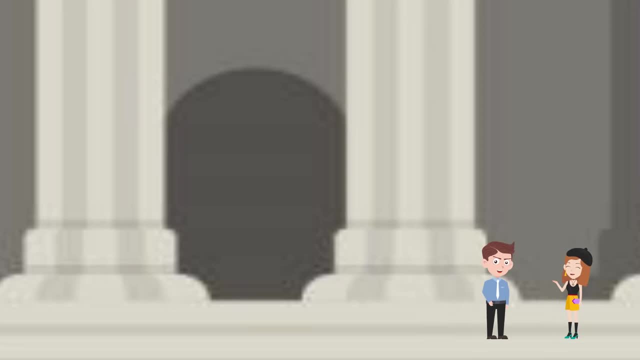 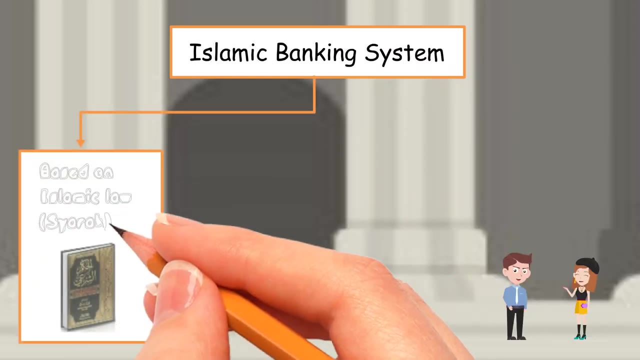 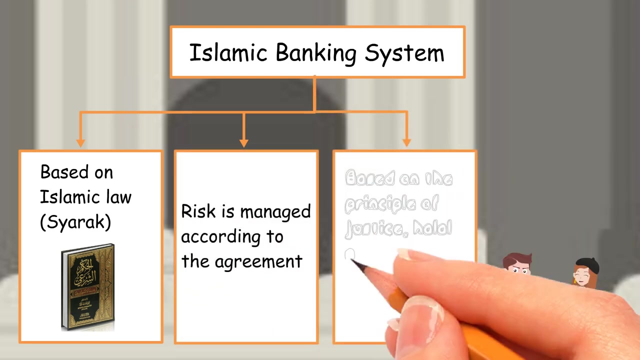 Yes, In Malaysia there are conventional banking system and Islamic banking system. Islamic banking system is based on Islamic law, Shah Raq. Risk is managed according to the agreement, Based on the principle of justice, halal profit sharing and without usury. 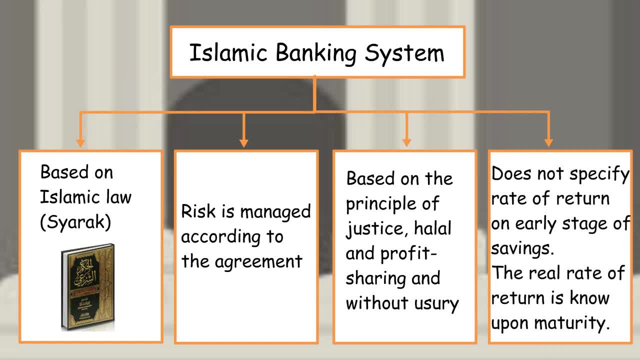 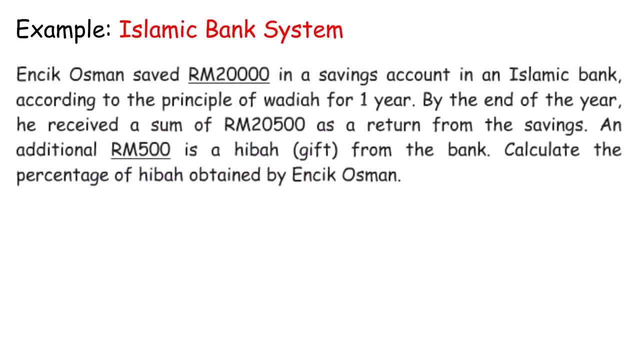 Does not specify rate of return on early stage of savings. The real rate of return is known upon maturity. Example: Ensik Osman saved RM20,000 in a savings account in an Islamic bank according to the principle of Wadia for a year By the end of the year. 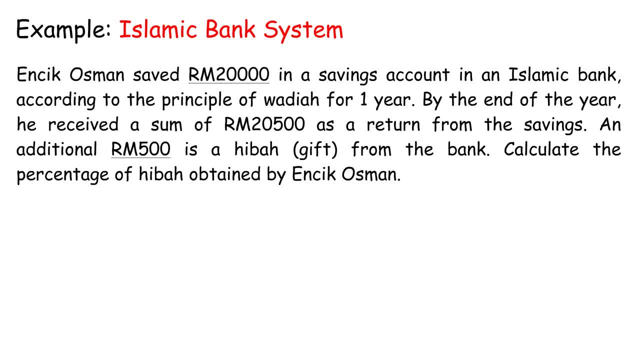 he received a sum of RM20,500 as a return from the savings. An additional RM500 is a IBA gift from the bank. Calculate the percentage of IBA obtained by Ensik Osman. Percentage of IBA equals RM500 over RM20,000 times 100% equals 2.5%. 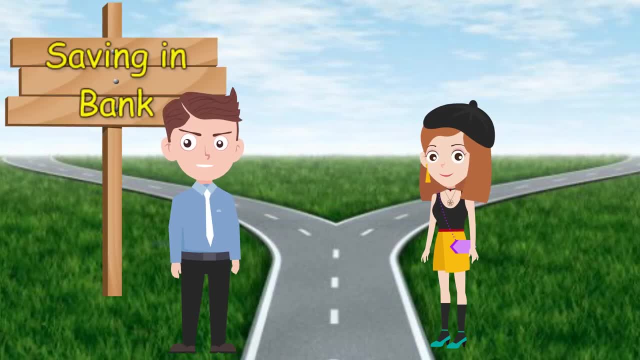 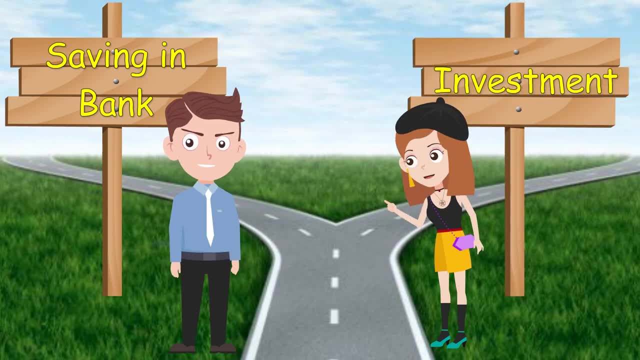 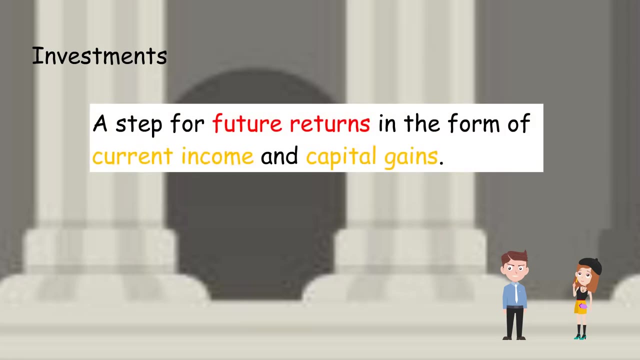 You can use your money to save your excess money in bank. You can use your money for investment. Investment- What is investment? This is the first time I hear this. It's OK, You will understand it very soon. Investment is a step for future returns in the form of current income and capital gains. 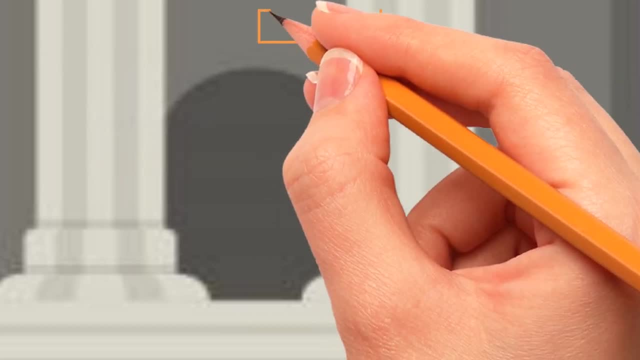 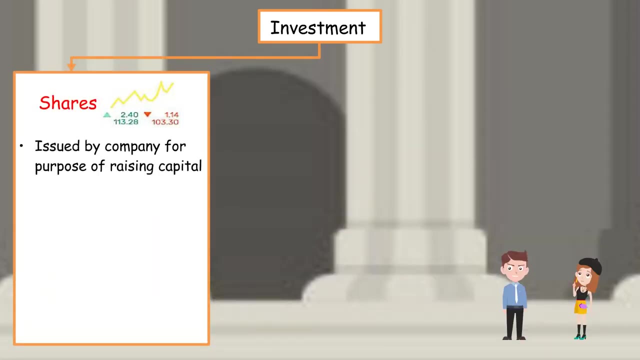 There are also three types of investment. First, shares: Shares is issued by a company for purpose of investment. Shares is issued by a company for purpose of investment, of raising capital. A person purchases shares from a company as the owner of the company under. 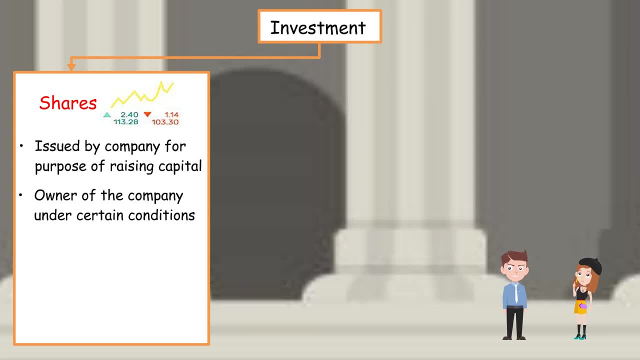 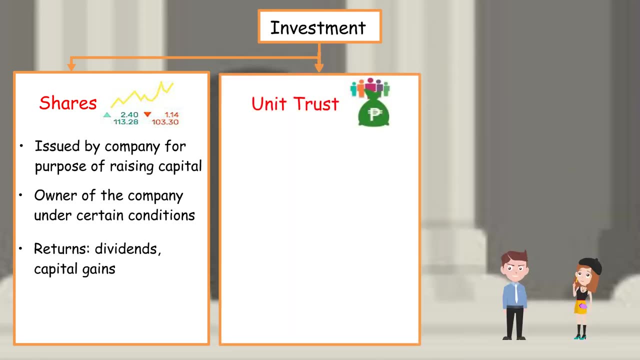 certain conditions, Shareholders will receive dividends and capital gains as returns. Second, unit trust Trust fund, controlled by a unit trust company managed by qualified professional manager in the field of investment, Collect money from investors and invest money in various potential companies with aim of providing returns that benefit investors. 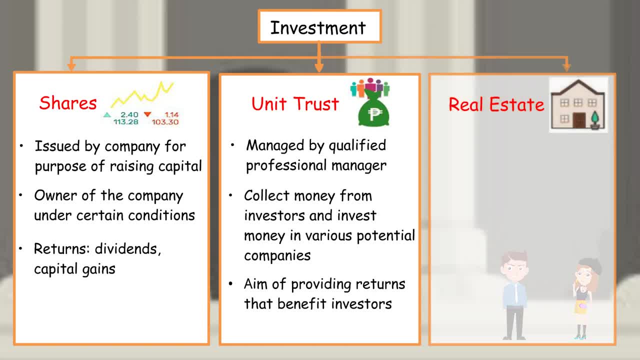 Thirdly, real estate Investments on immovable assets, For examples, houses, shops, land and others. Consider factors, economic situations, income generating capabilities, For example, rent location, property prospects in future, Receive investment returns in the form of renting and capital gains. 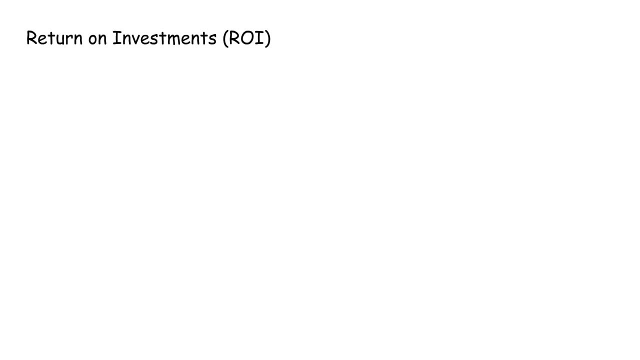 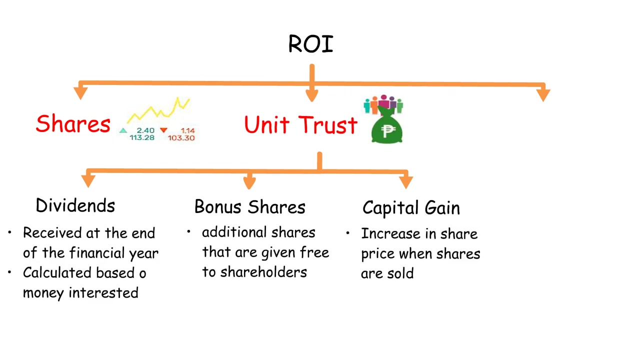 Now let me introduce you return of investment ROI. ROI is a ratio of profit or loss derived from an investment. ROI equals total return divide by value of initial investment times, 100 percent. The return of unit trusts are dividends, bonus shares and additional shares. Money handlerつまりaltra has your linings. What is your lease of assets? 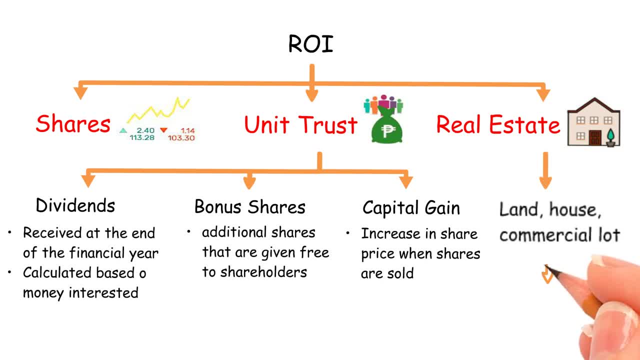 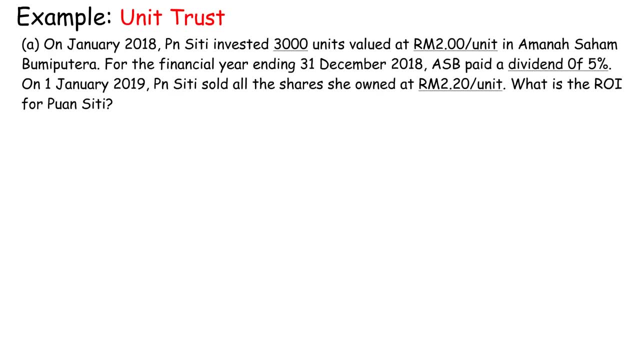 The return of investment. ROI is not just the initial investment, but both amount that looks like real estate and the additional interest group in the shareholder. This million-dollar dividend month isTs. So when you invest in a listing, it's about a requirement. 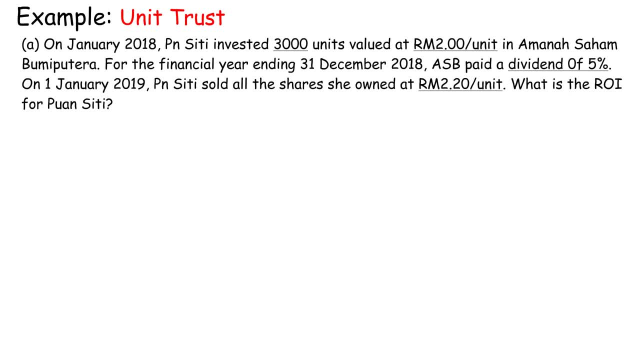 of 50 percent of that investment. Most of the investment you will get in the given year is interest and capital gains, But no risk of loss of funds remains 이야기able for the listing prices yourself. social device- Presentご input. You only have to do this in case of an emergency. Your listing is guaranteed for interest. 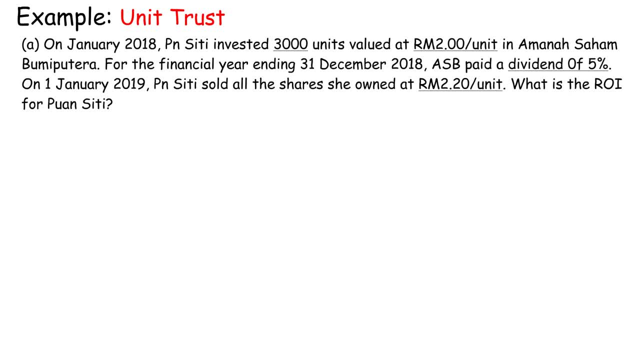 value. Value is as importantnies desarrollo and freelancing. Thank you for January 1, 2019, Puan City sold all the shares she owned at 2 ringgit 20 cent per unit. What is the ROI for Puan City? 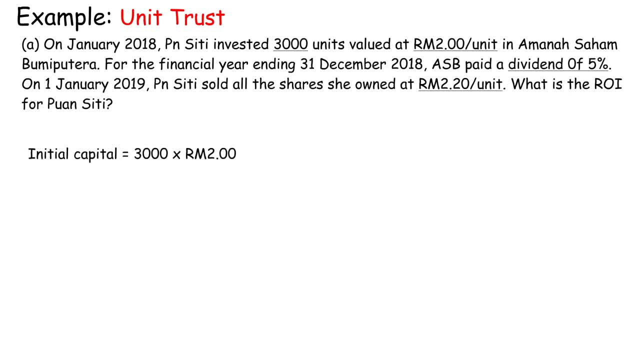 Initial capital equals 3,000 units times RM2, equals RM6,000.. Dividend equals 5% times initial capital Equals 5 over 100 times 3,000 units times RM2,: equals RM300.. Increase in share price: equals 2 ringgit 20 cent. minus 2 ringgit equals 20 cent. 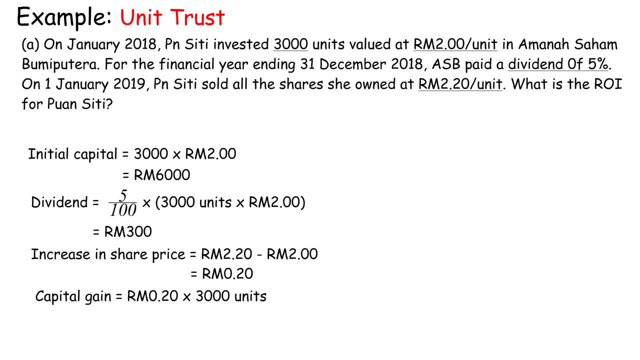 Capital gain equals 20 cent times 3,000 units equals RM600.. Total return equals dividend plus capital gain equals RM300 plus RM600 equals RM900.. To find out ROI, we need to write down the formula. ROI equals 2,000 units times 3,000 units times RM600.. 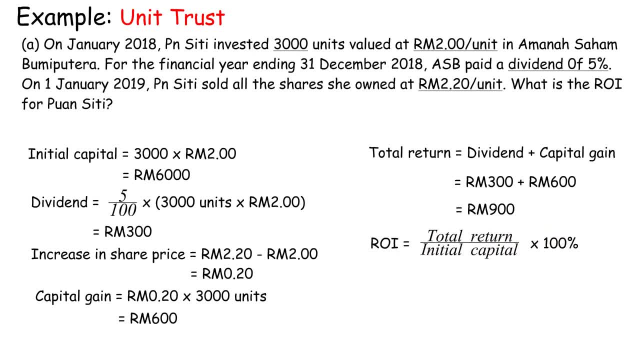 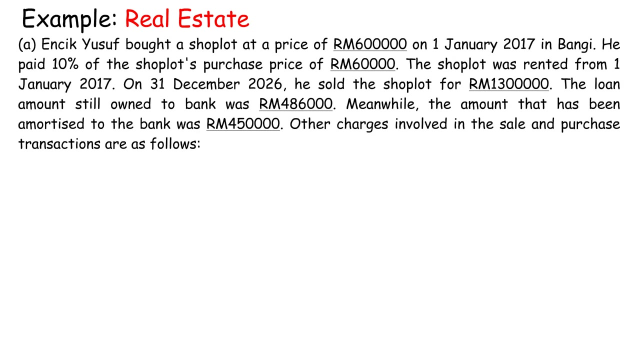 Total return divide by value of initial investment times 100% Equals RM900. divide by RM6,000 times 100% equals 15%. Therefore, the ROI for Puan City is 15%. For real estate example, A Encik Yusof bought a shop lot at a price of RM600,000 on January 1,. 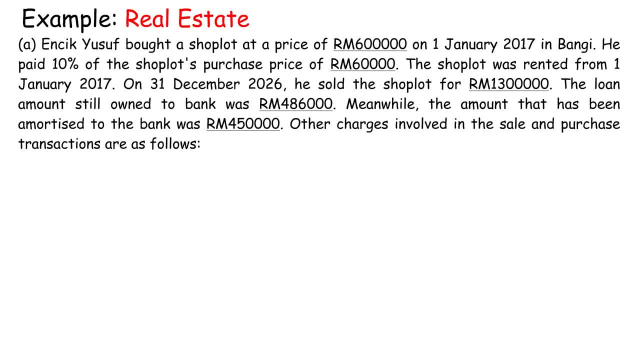 2017 in Bangui, He paid 10% of the shop lot's purchase price of RM60,000.. The shop lot was rented from January 1, 2017.. On December 31, 2026, he sold the shop lot for RM1,300,000. 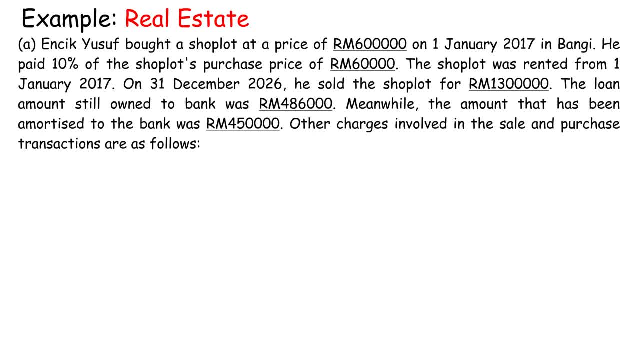 The loan amount still owned to bank was RM486,000.. Meanwhile, the amount that has been amortized to the bank was RM4,000.. Other charges involved in the sale and purchase transactions are as follows: Legit cost: RM15,000.. 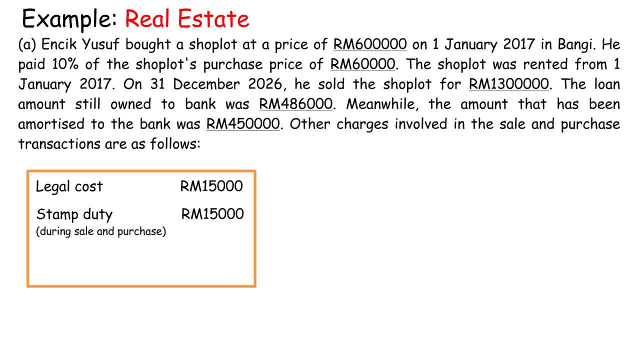 Stamped duty during sale and purchase: RM15,000.. Agents commission: RM18,000.. Total rent collected is RM200,000.. Calculate ROI obtained by Encik Yusof, Total rent equals RM200,000.. Capital gain equals RM1,300,000 minus RM486,000. minus RM60,000 minus RM15,000 minus RM15,000 minus RM18,000 minus RM450,000 equals RM256,000.. 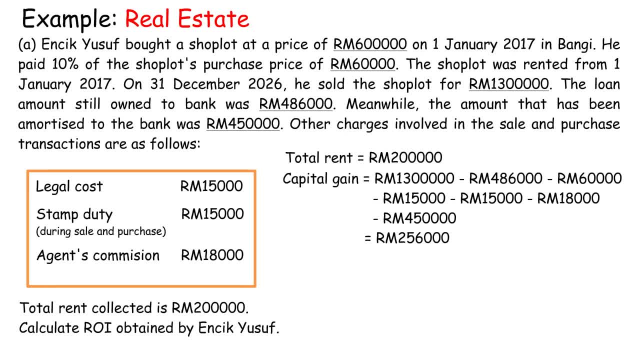 Total return equals total rent plus capital gain. Equals RM200,000 plus RM256,000.. Equals RM456,000.. ROI equals total return. divide by value of initial investment times. 100%. Equals RM456,000. divide by RM600,000 times 100%. 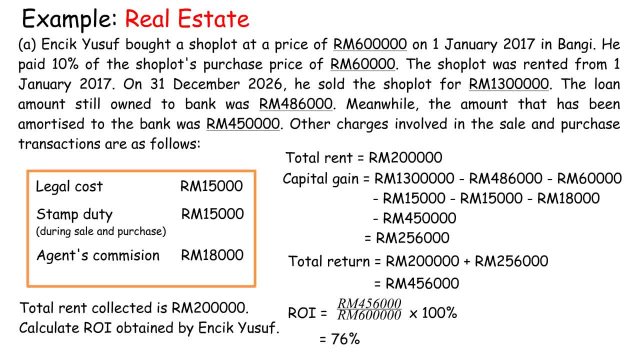 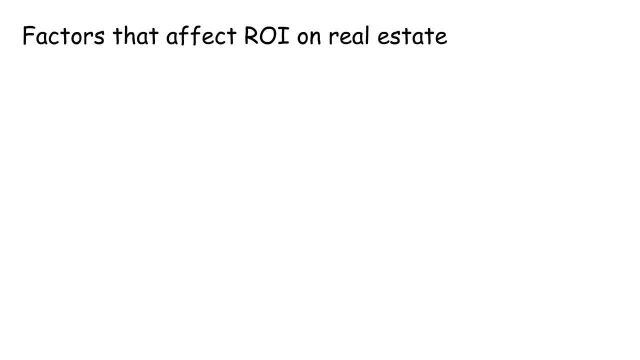 Equals 76%. There are some factors. There are some factors that affect ROI on real estate: 1. The economic situation: Country's good economic situation, demand will be higher and the real estate prices will increase. 2. Location: Properties located near a vastly developed city center have higher prices compared to properties in rural areas. 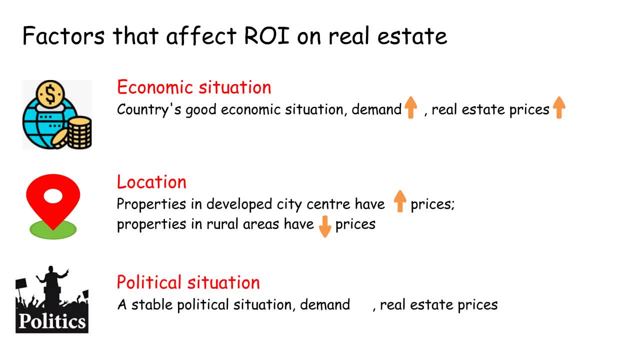 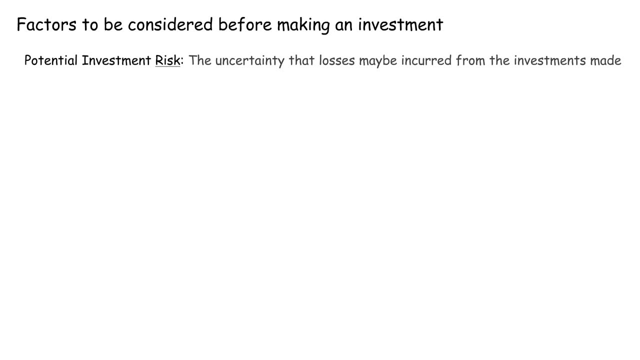 3. Political situation. 4. A stable political situation will increase demand and increase the real estate prices. Factors to be considered before making an investment: 1. Potential investment risk: The uncertainty that losses may be incurred from the investments made. 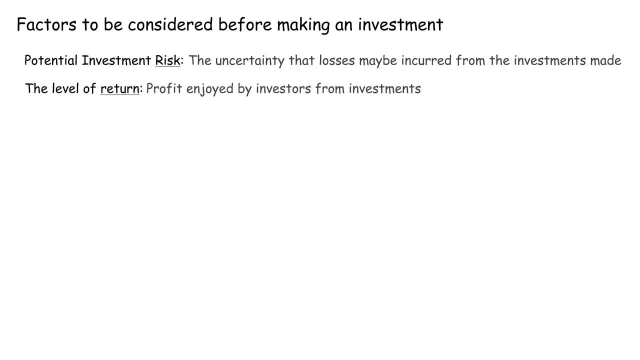 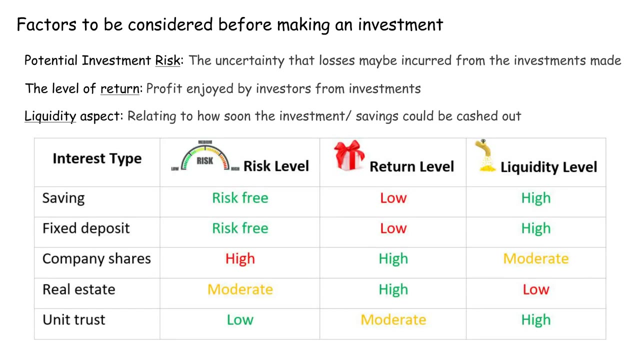 2. The level of return Profit enjoyed by investors from investment. 3. Liquidity aspect Relating to how soon the investment or savings could be cashed out. The summary table are shown as follow. There is a strategy called cost averaging strategy. 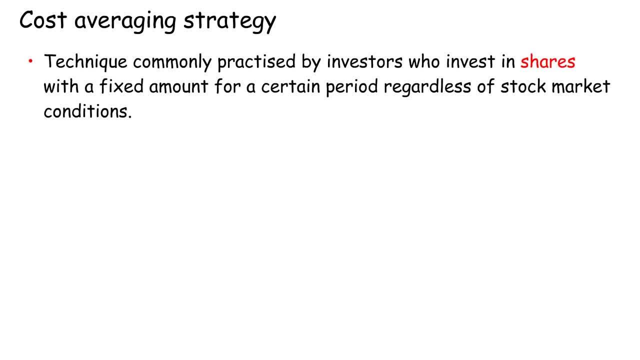 It is a technique commonly practiced by investors who invest in shares with a fixed amount for a certain period, regardless of stock market conditions. It helps investors to buy shares with a lower average cost. Total number of shares owned will be higher within the same investment period. 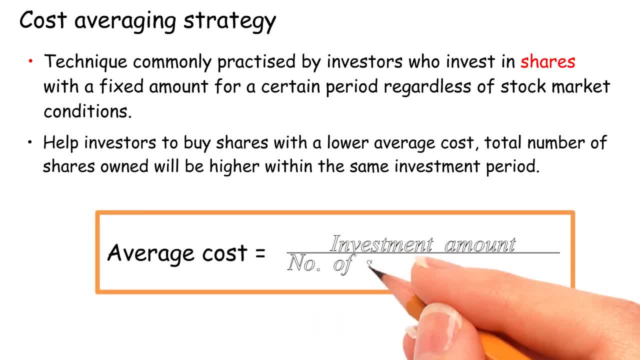 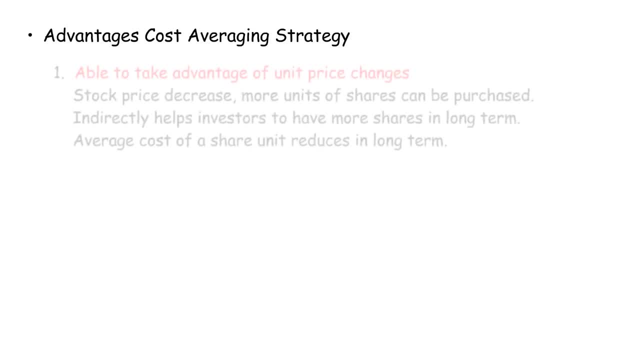 Average cost equals investment amount divided by number of share units owned. The advantages are: 1. Able to take advantage of unit price changes. Stock price decrease. more units of shares can be purchased Indirectly. helps investors to have more shares in long term. 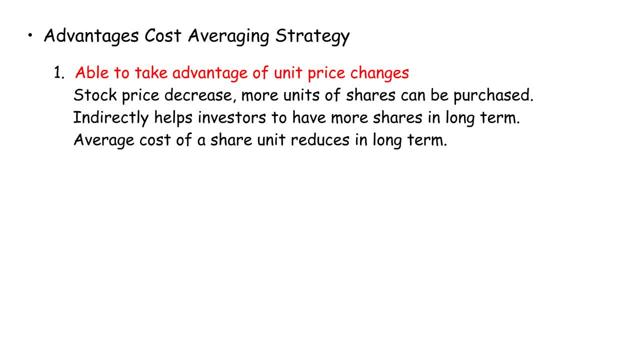 Average cost of a share unit reduces in long term. 2. Not influenced by emotions: Invest consistently, on a periodic basis, the same amount of money Without being influenced by emotions caused by share price fluctuation. 3. Lower the risk of loss. 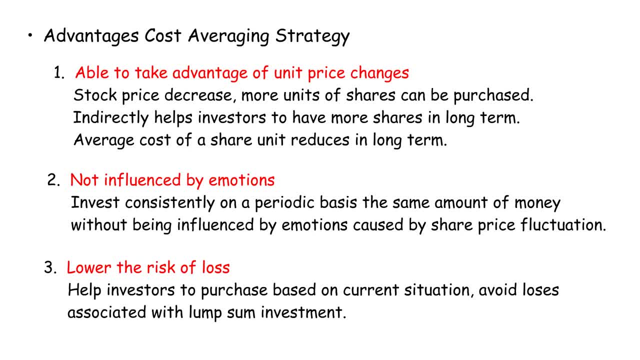 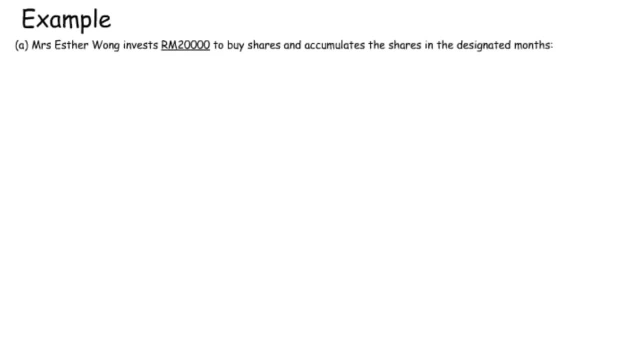 Help investors to purchase based on current situation. Avoid loses associated with loss. Avoid losing the chance of loss. Don't force investors to lose. It is essential that investors understand the agreed spirit of investors and use a standardized rules of conduct, thinking clearly with a clear mind. 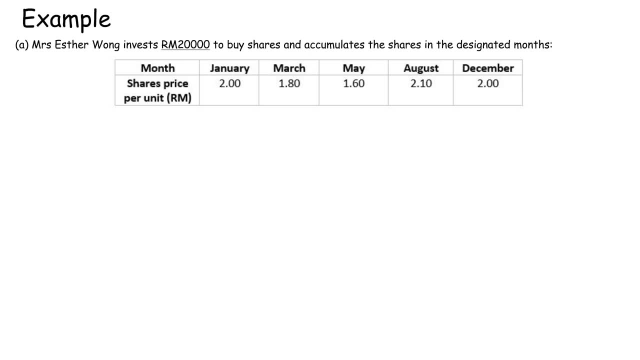 Concentrate yourself to many different factors. You need to know the parts of a share and discuss them thoroughly. Think carefully about the item you are investing. What you are investing is the real part of your investment. Calculate the average cost per unit and the number of shares owned by Puan Linda and Mrs Esther Wong. 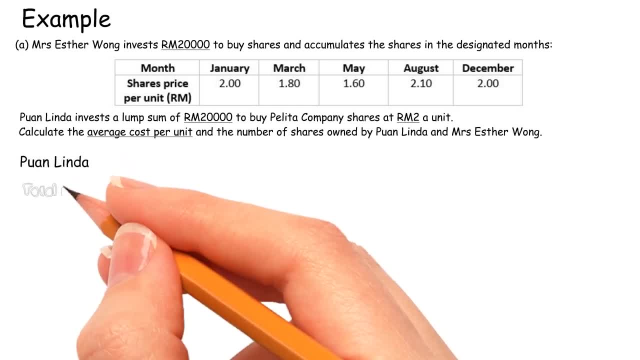 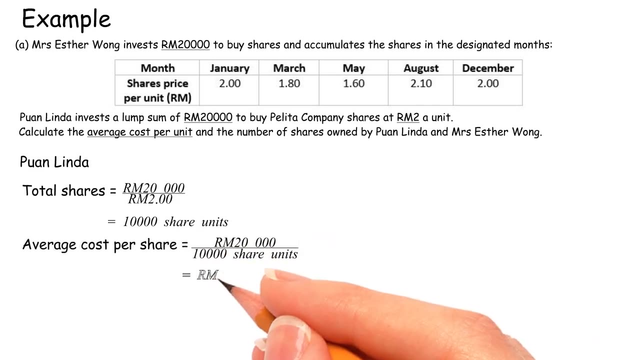 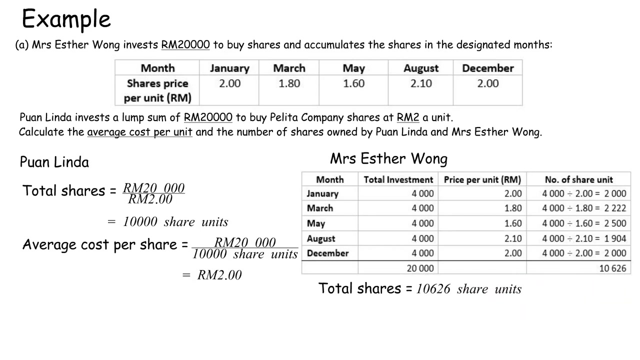 For Puan Linda, total shares equals RM20,000. divide by RM2, equals 10,000 share units. Average cost per share: equals RM20,000. divide by 10,000 share units equals RM2.. For Mrs Esther Wong, total shares equals 10,626 share units.